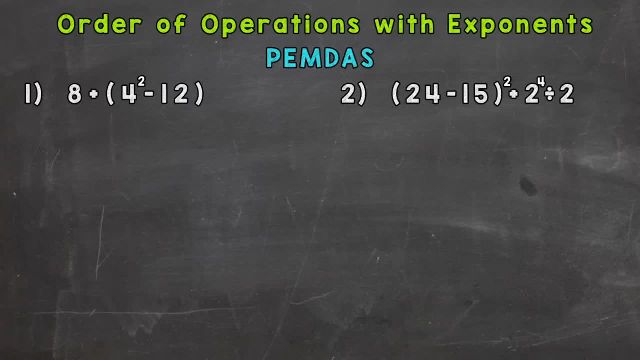 the top of your screen in blue, is a little reminder here of the steps we're going to take in order to solve these correctly. PEMDAS, the specific order in which we need to solve these problems, right Parentheses: priority number one, then exponents multiplication and. 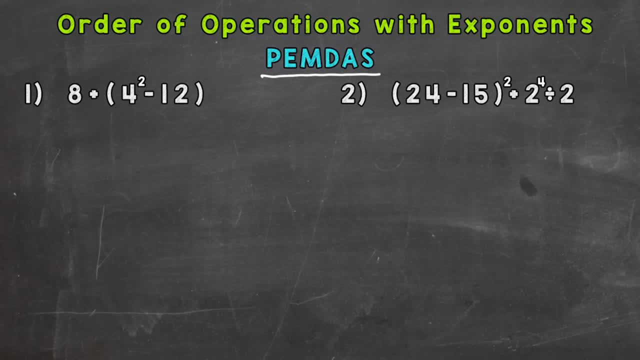 division and then addition and subtraction. So let's jump right into number one here, where we have 8 plus parentheses, 4 squared minus 12, and then end parentheses. So the first thing we need to take a look at is what's in the parentheses, And we have 4 squared minus 12.. So 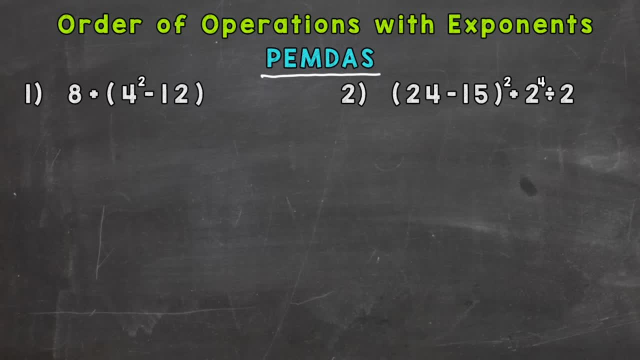 we have an exponent and we have subtraction, So that exponent holds the highest priority within the parentheses. So we need to do 4 squared first, which means 4 times 4, not 4 times 2,, 4 times 4.. So that equals 16.. I'm going to bring down everything else I did not use, And now we 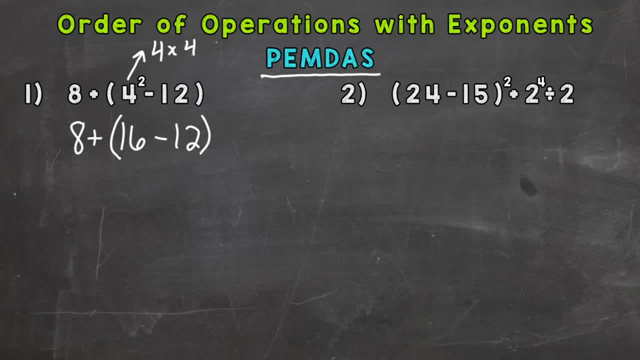 have 8 plus parentheses. 16 minus 12,. end parentheses, So parentheses again. we need to bring those down so they still hold the highest priority. So 16 minus 12, would give us 4. Bring down everything we did not use, which is just that 8, and the addition sign. 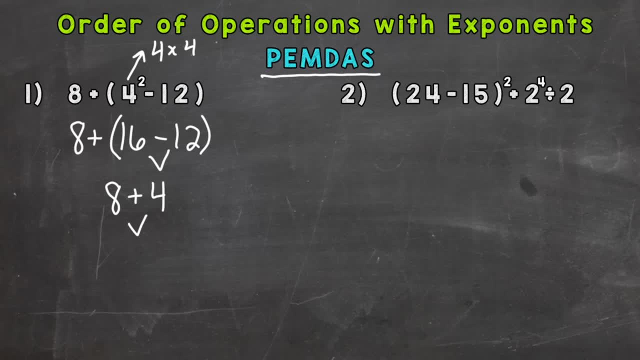 And then we wrap up the problem with 8 plus 4, which gives us 12.. So let's take a look at number two here, where we have 24 minus 15 in parentheses, And that whole thing is squared right. A power of 2 next to the parentheses. That just means we do. 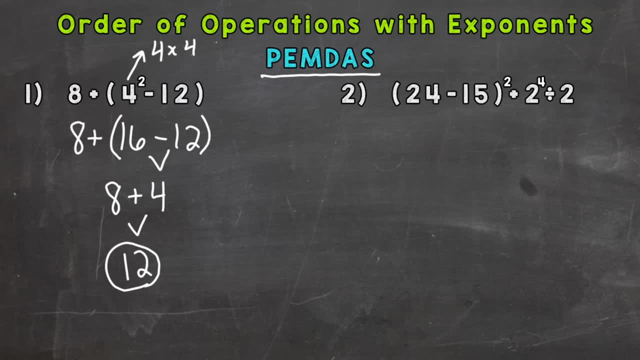 everything in the parentheses and then take it to the power of 2.. Plus 2 to the fourth power and then divided by 2.. So let's go through our steps. Are there any parentheses in this problem? Yes, So, highest priority, we need to do that first. 24 minus 15 gives us 9.. Now that used up. 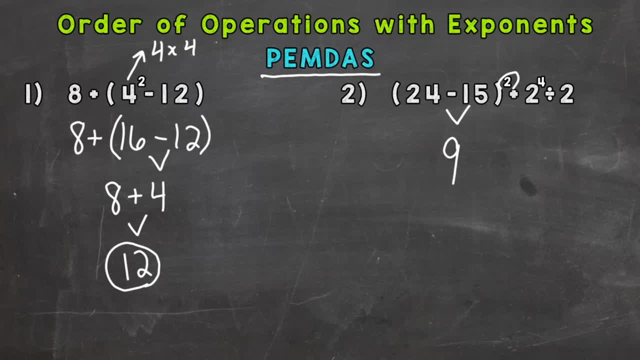 everything in those parentheses, but we need to do that again. So 24 minus 15 gives us 9.. We still have to the power of 2.. So that's attached to whatever our answer is from inside those parentheses, And I'm going to bring down everything else we didn't use as well. 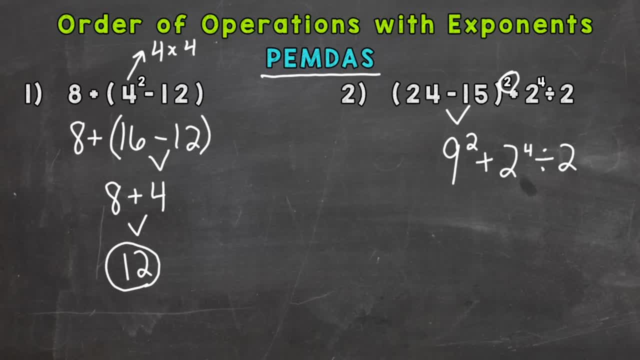 So now we still have a bunch of stuff going on. We have a power of 2, a power of 4, an addition sign and a division sign. So let's go through our steps and start breaking it down further. Are there any parentheses? No Exponents. Yes, We have 2.. The power of 2 and the power of 4.. 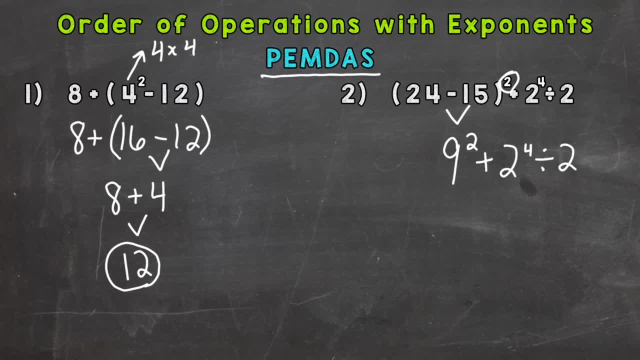 So if you ever have 2 or more of things that are on the same level, right, So we have 2 exponents there, So they're of the same priority. You go left to right, So we're going to do the 9. 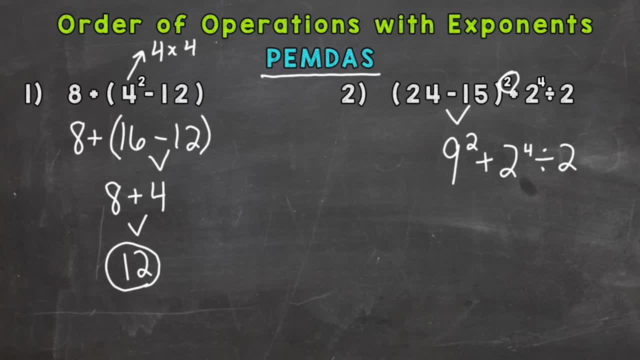 to the second power first, which gives us 9 times 9, which is 81.. Bring down everything else we did not use. So addition to the power of 4 and division. So any parentheses No, Any exponents Yes. So we need to do the exponents 2 to the fourth power, which is not 8.. It means 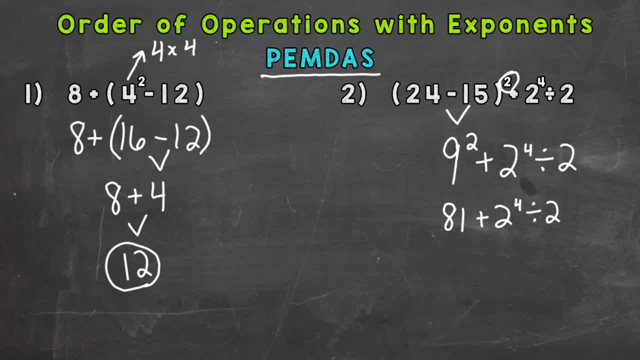 2 times 2 times 2 times 2.. Well, 2 times 2 is 4.. Times 2 is 8.. Times 2 is 16.. Bring down everything I did not use. And now we have it narrowed down to addition and division. So any parentheses No. 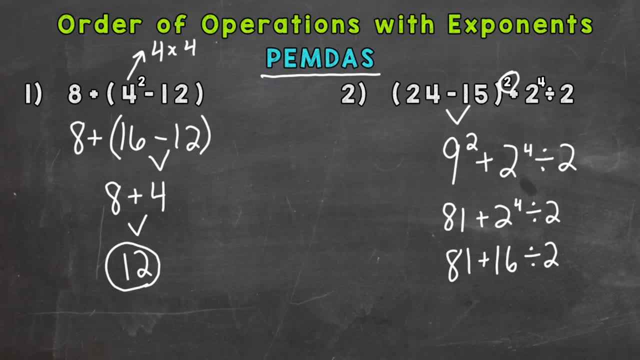 Exponents: No Multiplication or division. Yes, We have 16 divided by 2.. So that would be next priority, And 16 divided by 2 is 8.. Bring down our 81 and the addition sign And we're down to our. 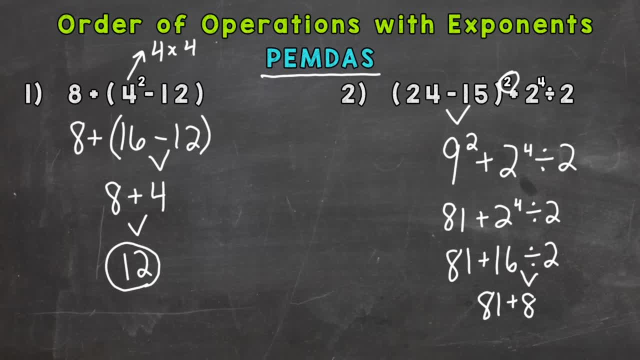 addition problem 81 plus 8, which gives us an answer of 89.. So there you have it. There's a couple of examples of order of operations, problems with exponents, And there's also parentheses in there as well. So I hope that helped. Thanks so much for watching. Until next time, peace. .